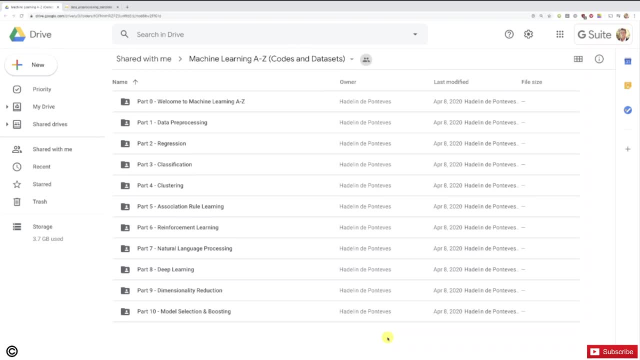 rules inside an ensemble of transactions- All right, so very useful, especially for retail businesses or any kind of e-commerce. So if you are a data scientist working for an e-commerce company, you will definitely use it, and if you are yourself, you know- a business owner of a retail company or 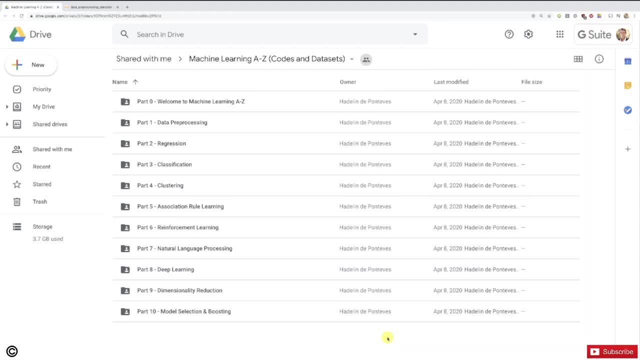 an e-commerce company, then you will definitely benefit from it as well. All right, so let's do this. Let's start to learn this new part of association rule learning. So let's start to learn this new technique. and before we start, let's just make sure everyone here is on the same page. 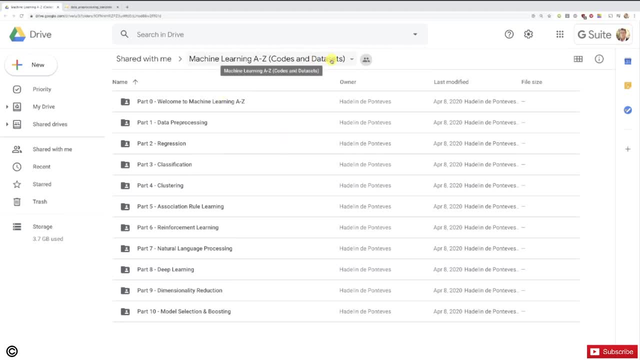 This is a folder containing all the codes and data sets of this course, and I gave you the link to this folder right before this tutorial, so make sure not to miss it. Click it, and now we should all be on the same page. All right? so let's do this. Let's get into part five: association rule. 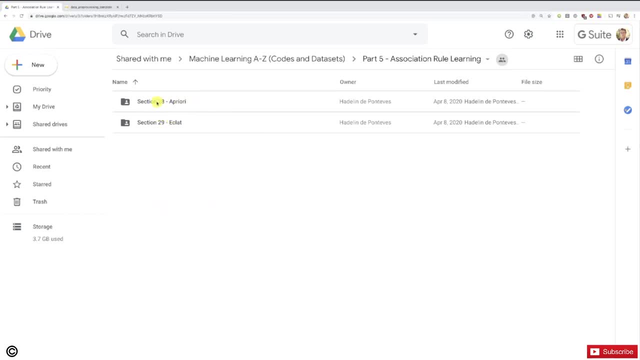 learning, and we are going to cover two models: The first one, a priori- which is actually the best one of the two, if you want my opinion- and ECLA. and of course, we're going to start with a priori and we're going to start here with python. All right, so inside this python folder, 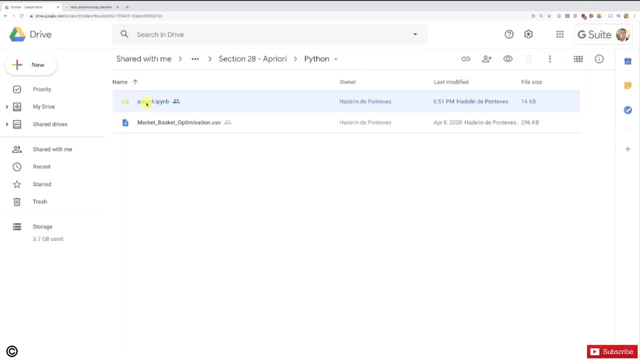 you will find, as usual, the implementation, a prioriipynb which you can open with either google collaboratory or jupyter notebook and, of course, you will find the data set, which is called market basket optimization, because actually association rule learning is used to do market. 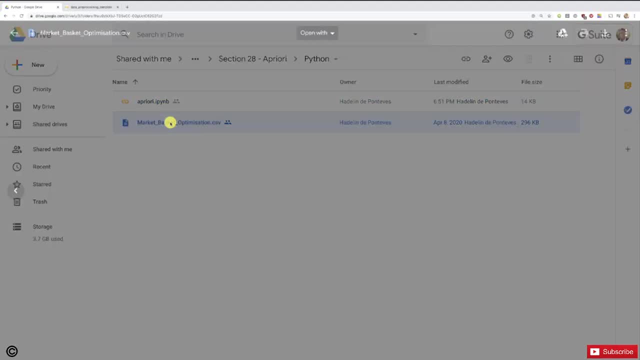 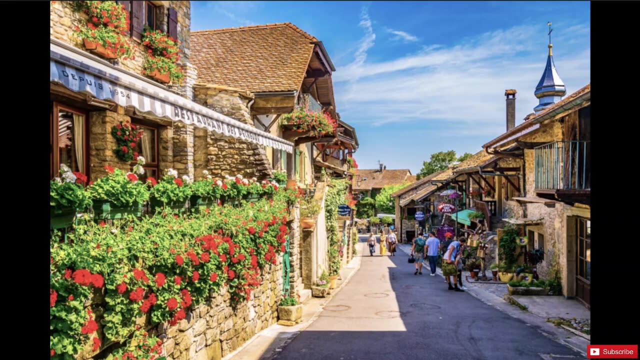 this way. All right, so, speaking of which, let's describe what this data set is about. All right, so, for starters, let's imagine the beautiful region of south of France, you know, with all these cute villages, with happy people walking down the streets and going to the grocery store every. 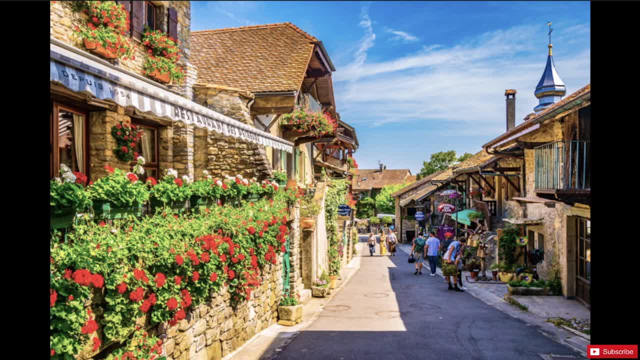 now and then, or to the coffee places. Well, you know, imagine a very lively place where people hang out a lot and love going to the different shops, the different commerces, not only to buy their favorite products but also to, you know, chill out in the beautiful lovely. 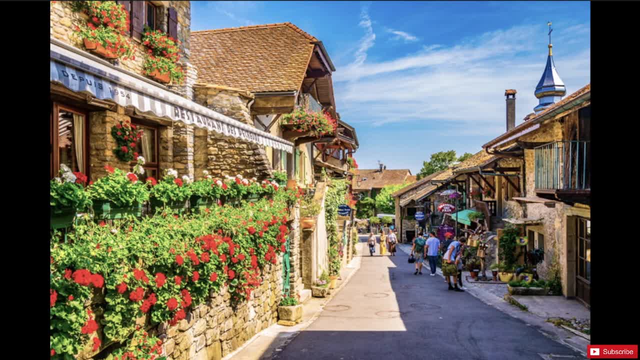 town and imagine that you are the business owner of one of these stores. you know selling food and delicious stuff, and so you know you are the business owner of this shop and you would like to, as any business owners, optimize and boost the sales. and you have an idea: it is to offer some. 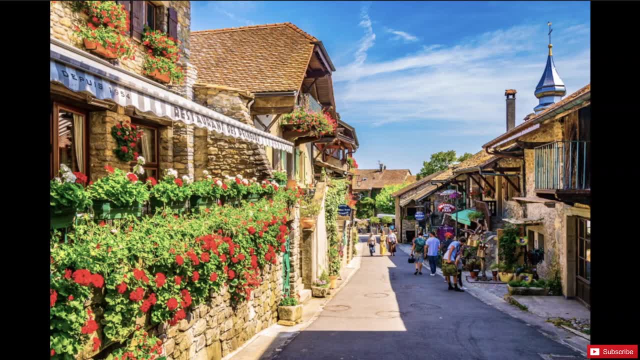 new, great deals to your customers, and the deal idea that you have in mind is to identify, you know, the best association rules among the different products bought by your customers in order to offer, you know, this very famous deal: buy this and get that for free. you know, if you buy this product, you're gonna get that product. 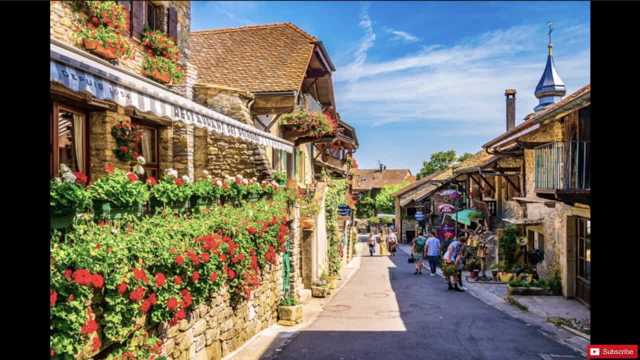 for free. all right, and so now you see the idea. we're gonna use association rule learning to find the strongest rules, saying if customers buy this product, then they will have a high chance to buy that other product. and we will measure that chance so that, in fact, if they get this product, 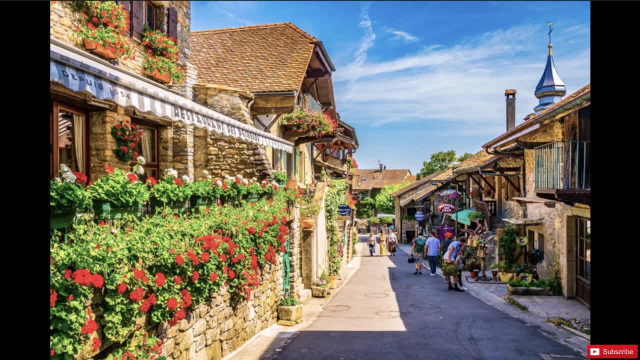 they will very likely want this other product and therefore they will very likely get that deal: get this product and they will be able to buy that other product, and they will be able to buy that and get that one for free. all right, so that's what this owner would like to do, and this owner just 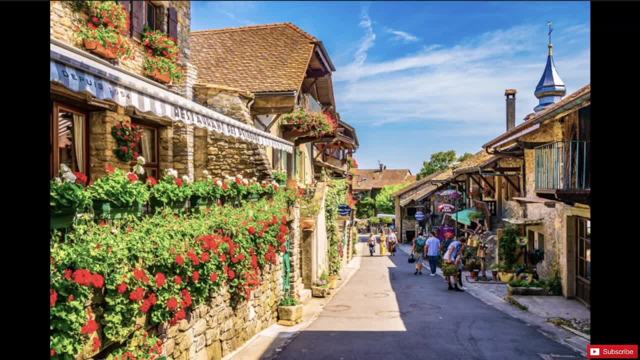 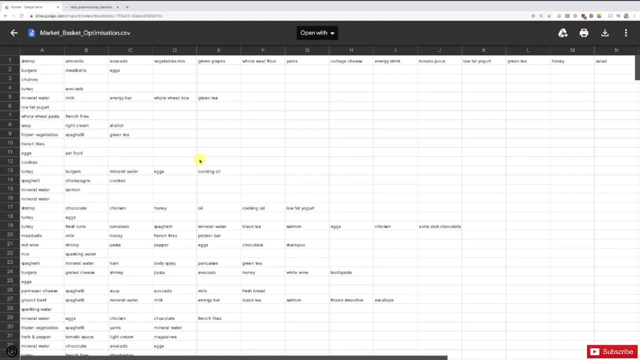 hired the best data scientist of thousands of friends, which means you, of course, to do the job you know, to find these association rules and therefore what this owner did, because he knows a little bit about data science. he knows that he has to collect some data to provide to the data. 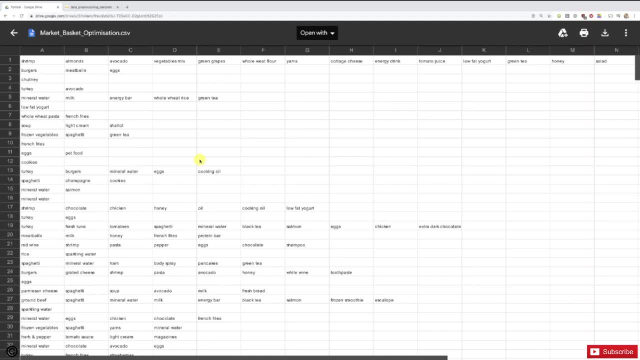 scientists in order to learn these rules, and so, each week, this owner collects all the different transactions of the customers and at the end of the week, you're given this list of transactions which you have in front of you, so that you can learn the association rules and return the best. 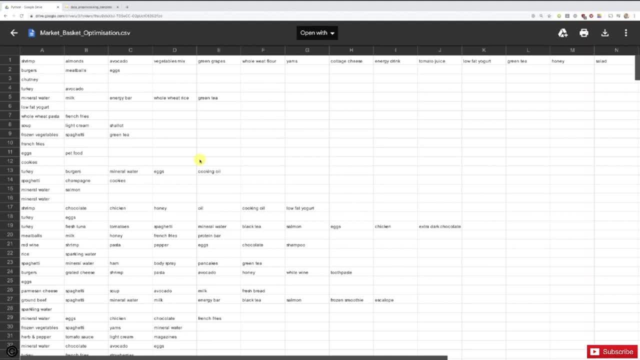 deals that this owner should offer to the client. all right, so that's your mission: you have to identify the best deals so as to maximize the chance that you know the customers will get the deals. you know we'll buy this product and get another one for free and, of course, the price of 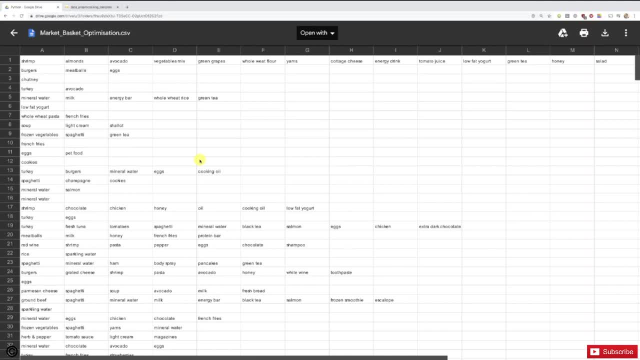 this buy this, get one for free- will be well calculated by the customer, so that you can buy the owner- but that's a different question- so that it can indeed not only optimize the sales but also the profit. all right, so that's the mission, and now let's make sure everyone understands the 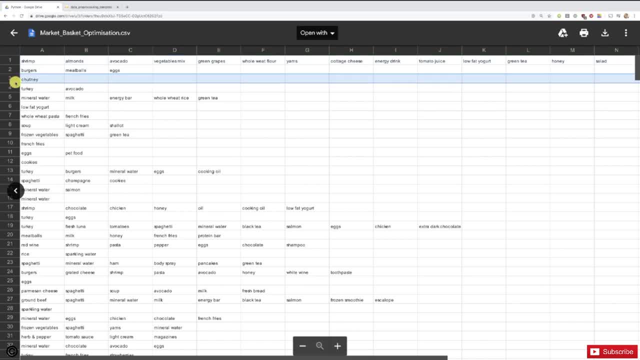 data set. you know each row of the data set corresponds to different transactions, you know, from different customers actually, and for each of these transactions you have all the different products that the customer who did the transaction purchased. all right, so, for example, this first transaction corresponds to a certain. 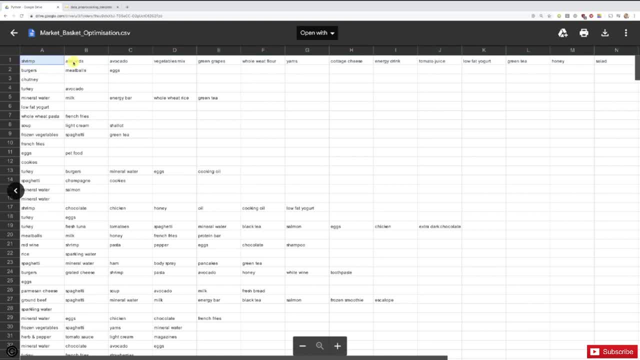 customer who bought in one basket some shrimps, some almonds, avocado, vegetable mix, green grapes, Etc. up to you know olive oil. all right, then this customer, or you know this transaction, corresponds to a customer who bought in one same basket some burgers, meatballs and eggs. all right, this customer. 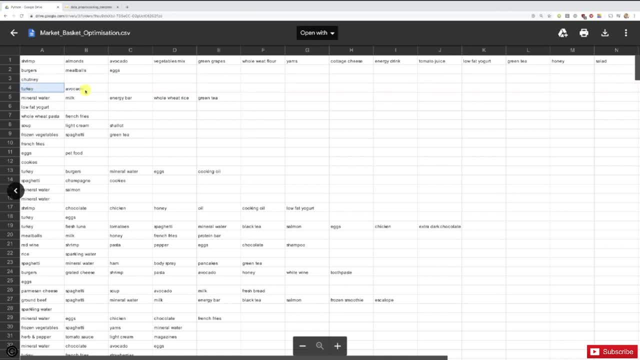 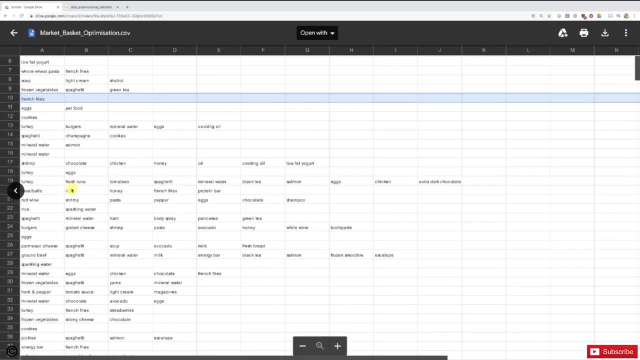 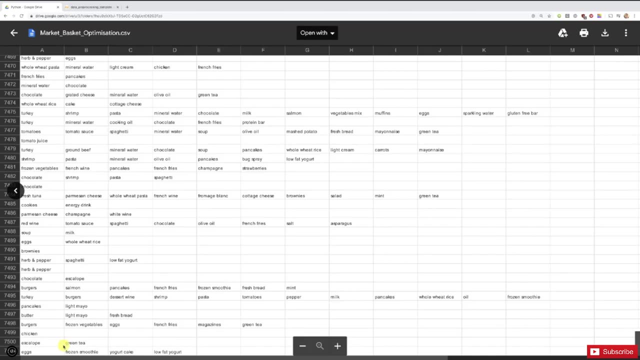 just bought chutney. this fourth customer bought turkey avocado and Etc. right, so all these transactions correspond to different customers and all these different transactions- there are actually many of them, they're actually 7 500, you know, if we scroll down up to the end, yes, 7 500. and these 7 500 transactions were collected during the 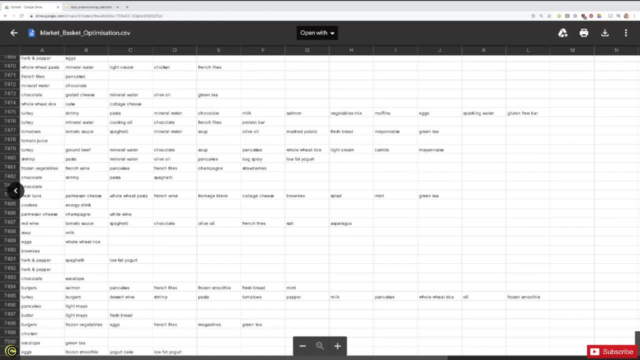 whole week. you know, each week the owner of the shop does this. he records all the transactions and he gives them to you, data scientist, so that you can learn the association rules. all right, and your mission is to return to this owner as fast as possible. well, the best Association rules. 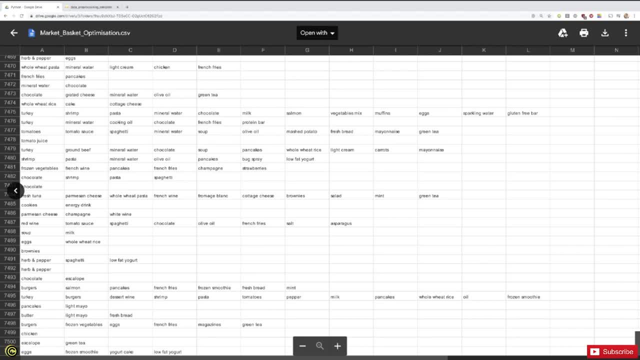 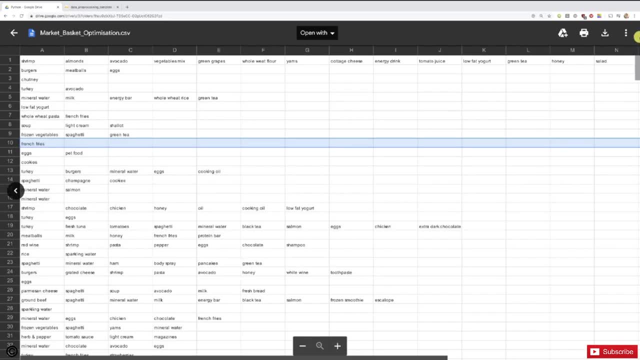 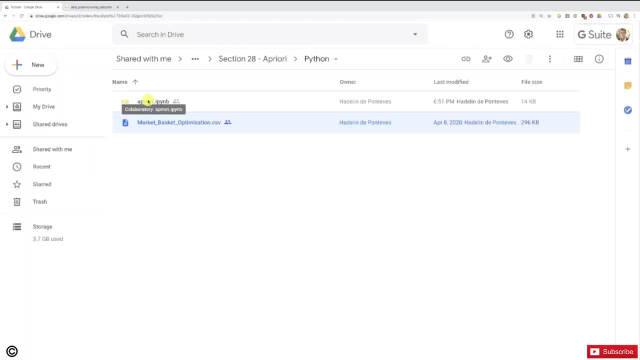 have two elements so that this owner can find the best deals for his clients. all right, good. so now that we clearly understand the data set, well, I suggest that we move on directly to the implementation. so we're going to go back to our folder and we're going to open this, a prioryipynb, either with 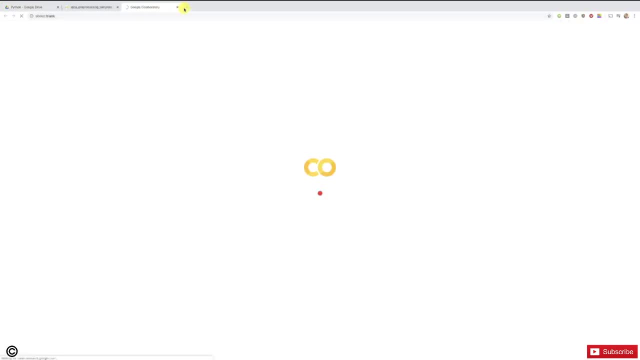 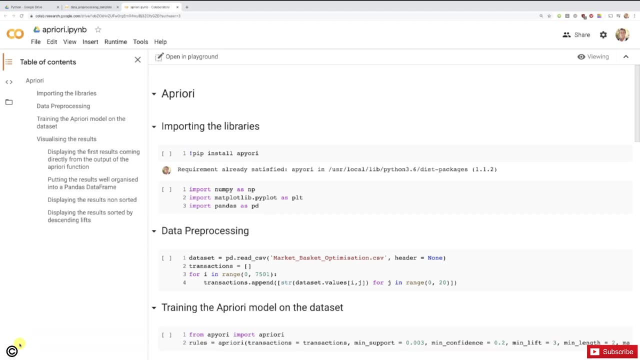 Google, collaboratory or Jupyter notebook, as you want, choose your favorite. now it is loading, it is laying out the notebook and in a second we'll have it opened. all right, perfect. so, as usual, this notebook is in read only mode, and therefore what we're all? 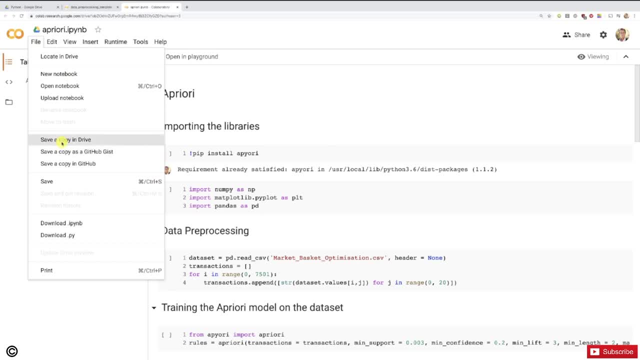 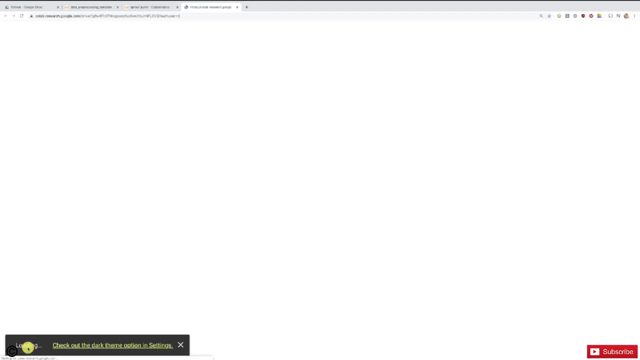 going to do now is go to file here to create a copy. by clicking here on save a copy in drive, this will create a copy inside which we will be able to re-implement that file from scratch. all right, because I remind that this course is an action-based course, I want all of you to learn. 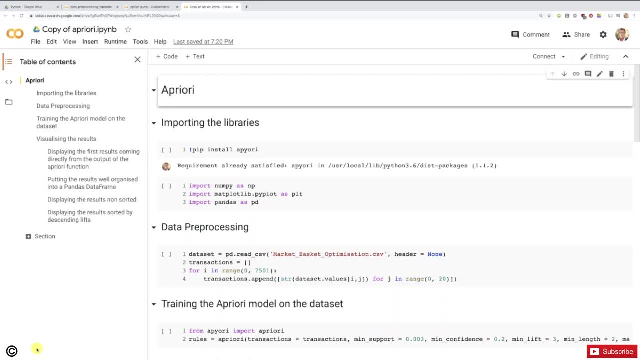 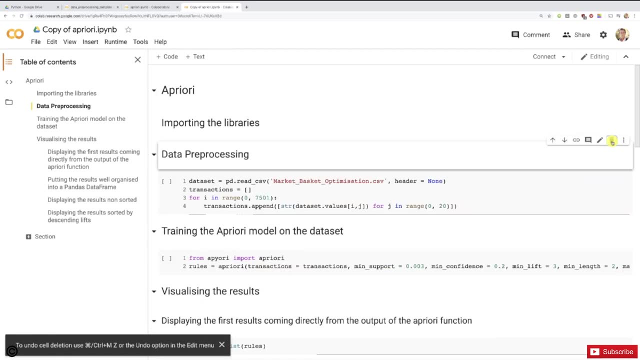 by doing, because this is how you will maximize your progress in machine learning. okay, so now again, as usual, let's remove all the code cells. you know, only the code cells, so that we can keep the well-highlighted structure of this implementation. so don't remove the text cells.